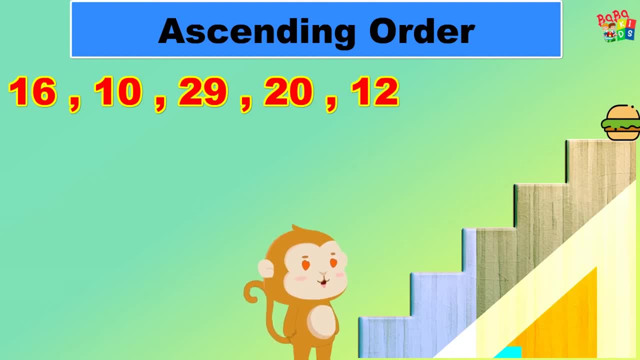 and 12.. They are not in ascending order, Children, if Mr Chiku wants to go up and get a burger, but for that the numbers should be arranged in ascending order. So, children, let's all have Mr Chiku to go upstairs and 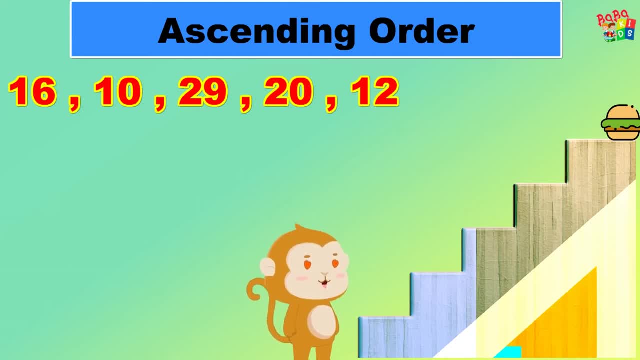 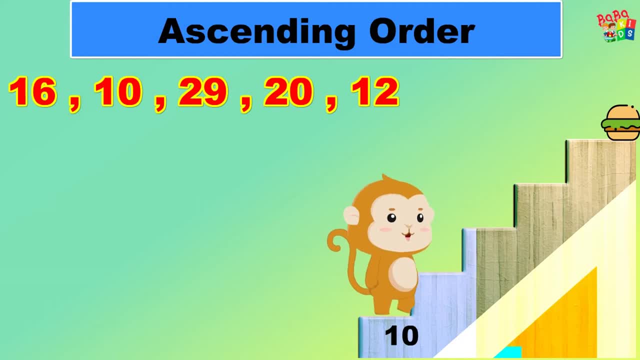 So the smallest number is number 10.. Then comes number 12.. Next is 16, followed by number 20.. And lastly number 29.. So finally, Mr Chiku got his burger. Now. smallest number is 10.. Then greatest number is 29.. 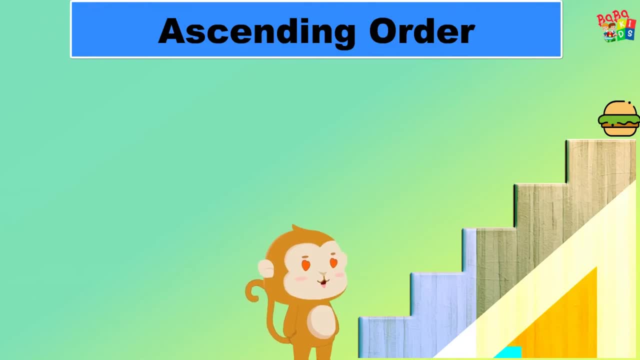 Now let's arrange another group of numbers in ascending order: 32,, 31,, 29,, 33 and 30. Now Mr Chiku wants again to get his burger. by arranging the numbers in ascending order, These given numbers, the smallest number is 29.. And next number 29.. 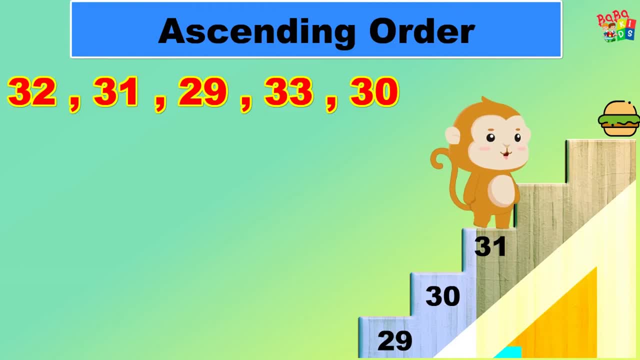 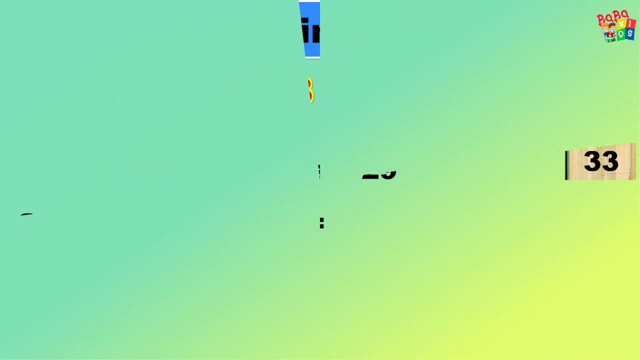 Then 31.. Then number 32., Then 33.. He got his burger. Smallest number is 29.. Biggest number is 33.. Now descending order. Descending order means arranging numbers from big to small, Or when we move from upstairs to downstairs is called descending order. Now descending order means arranging numbers from big to small, Or when we move from upstairs to downstairs is called descending order. Now, descending order means arranging numbers from big to small, Or when we move from upstairs to downstairs is called descending order. Now children: after eating burger, Mr Chiku wants to go back home. 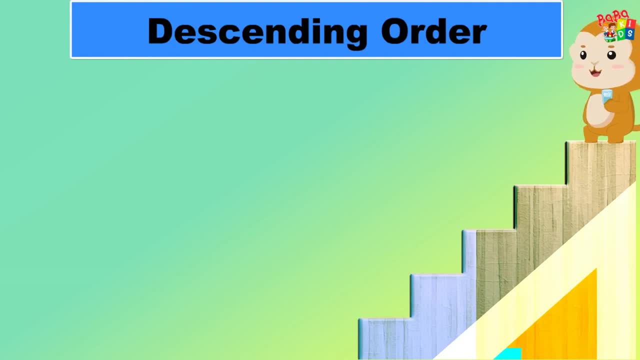